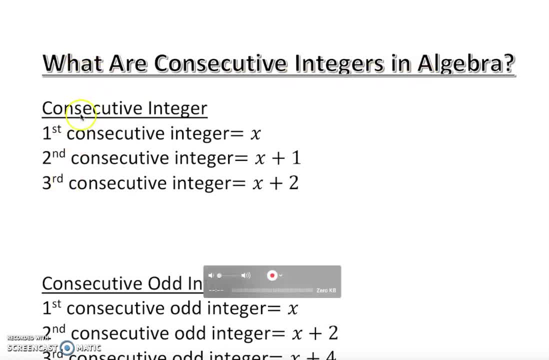 okay, let's talk about consecutive integers in algebra. so you know, in arithmetic, we know what is consecutive integers, right? so for example, let me actually explain you here. right, arithmetic, you know consecutive integers is basically like we can say one, two, three, four. these are basically consecutive integers, one after another. it's just one after another. if i say two, four, six and so on. 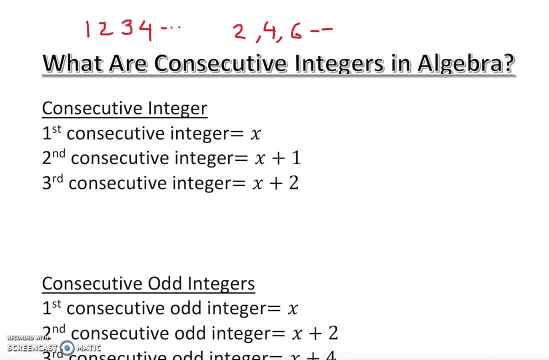 this is also consecutive integers, but what kind of integer it is is called even even right now there is another set: one, three, five, seven, and we call it what hard integers? okay, so these are basically what arithmetic now in terms of algebra, right? what are the consecutive integers? 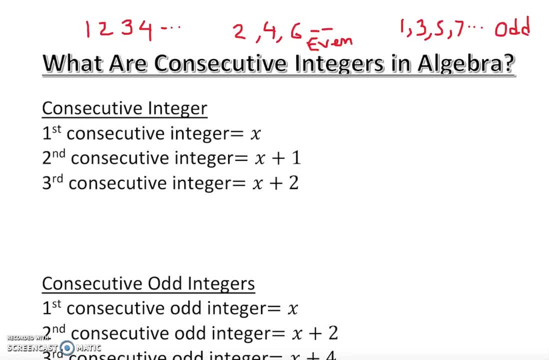 in algebra. so the first consecutive integers, as you clearly see here is going to be the x. well, why is x? because algebra is unknown. right, algebra is unknown, you have to know it, you have to find it. so first consecutive integer says always x. okay, well, or any variable i would. 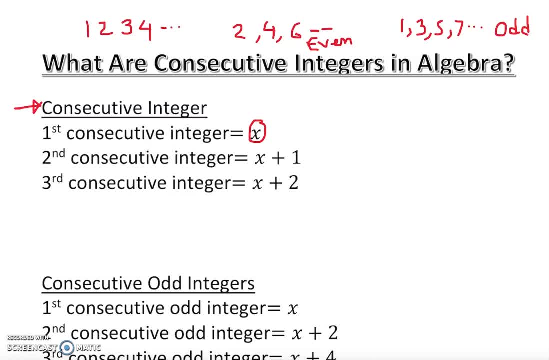 actually refer any variable. okay, i shouldn't say x, but any variable would find any unknown. okay, second consecutive is x plus one. third consecutive is x plus two. okay, so how do you know? this is what the answer is. let's verify it. actually, give me a number in your choice. okay, you're saying five. 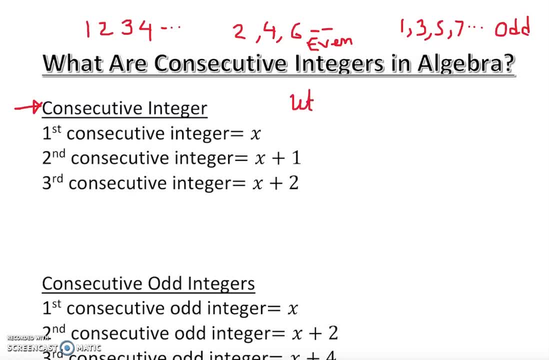 all right, let's let x equal to five. now inspect it. x equal to five. you're saying x equal to five, so five plus one, this gives you six and that's four. over here also, you're saying five plus two, because you said x equal to two, so it's going to give you seven. now have some observation. 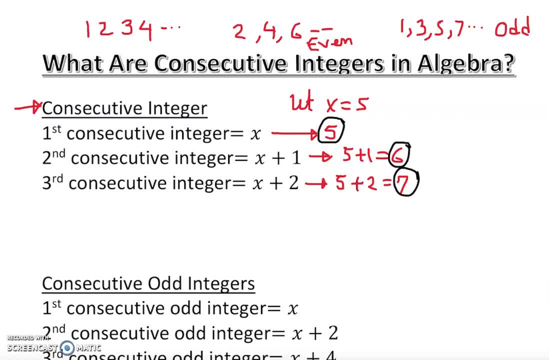 isn't it? consecutive integers, one after another. you found, see that. so this is called consecutive integers. now i'm going to do another example here. okay, i'm going to do another example. i'm going to say: let's give me another example. okay, let x equal to what you got, 20. okay, let's keep 20.. all right, 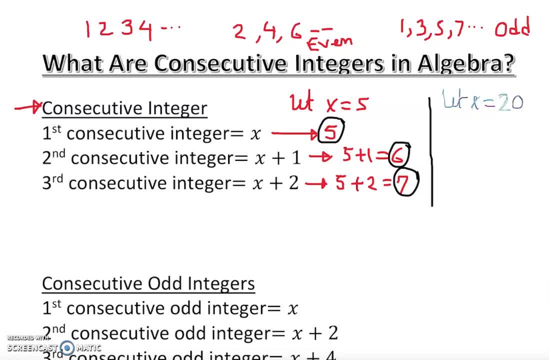 so let's make it more visible: 20.. okay, so we have a 20.. let's take a look here. so i'm going to have x equal to 20.. the first one, x equal to 20.. the next one, next consecutive integer, so you know x. 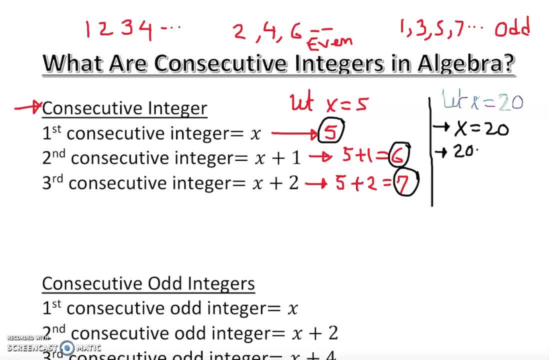 plus 1, so 20 plus 1, which is going to give you 21, and next one you're going to have x. you will assume x equal 20, so 20 plus 2, which is 22.. in other words, i can actually do it here instead of writing x. i can even put down: 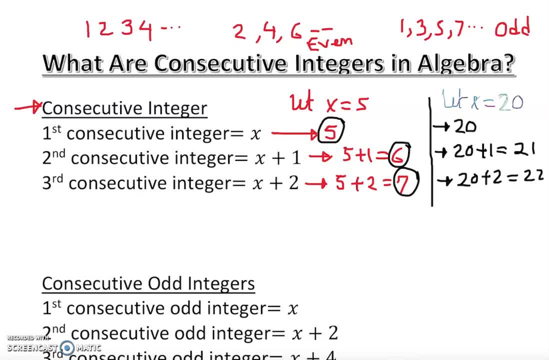 20 right here. okay, so you can see the differences. so that is the first outcome, because you assume this is your 20. you are picking up a number 20, next one gives you 21, the following gives you 22.. guess what? one after another. so those are consecutive integers. okay, so that's how you know. 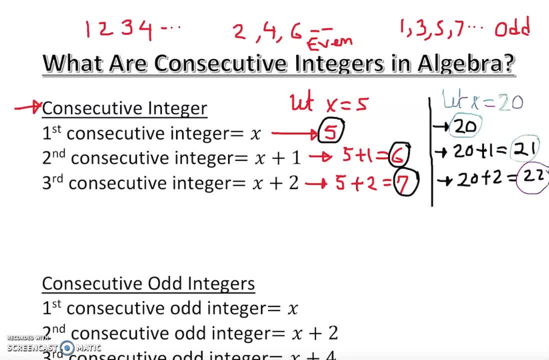 your consecutive integers in algebra. first one is x. usually many textbook they use x, x plus 1, x plus 2 and based on that you do have some application problem. another video i'm going to come up with the application problem like: find the sum of three consecutive integers. find the sum of two. 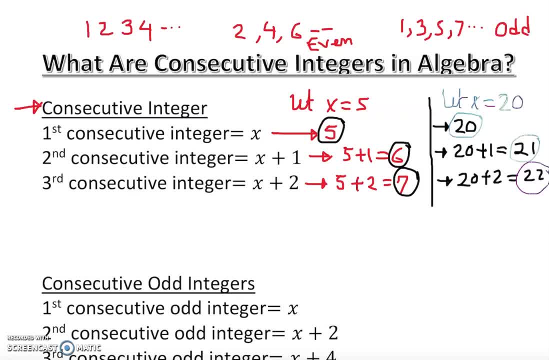 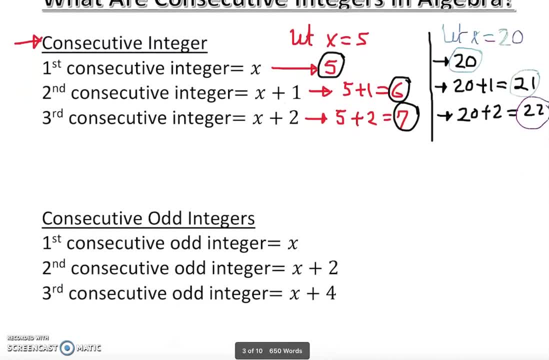 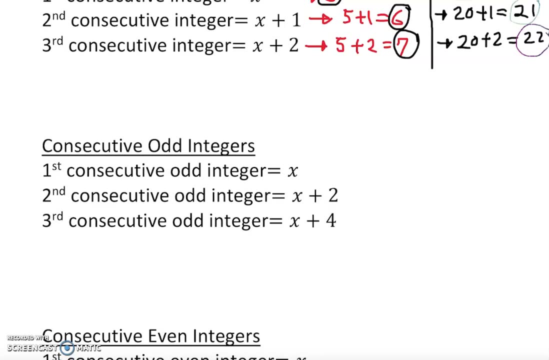 consecutive integers. okay, many, uh many, um, grade level: right algebra, this question is there. okay, so let's actually move into the next set. all right, so this is consecutive odd integer. so you kind of have a little bit feeling. what about the odd integers i just explained earlier? right, odd means one, three, five and so on. now give me a. 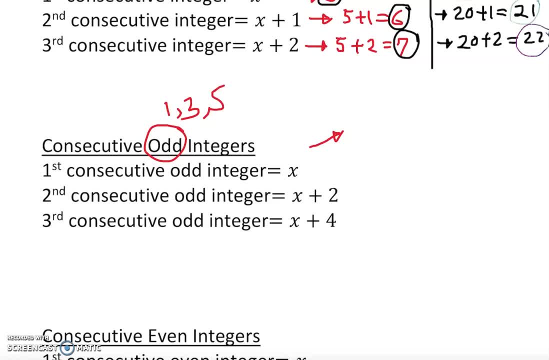 number. please give me a number, any choice. what nine? okay, you said nine, so let x equal to nine. okay, so i'm gonna say x equal to nine, and over here i'm gonna say nine plus two, which is eleven, over here i'm gonna say nine plus four. some you say: how do you come? 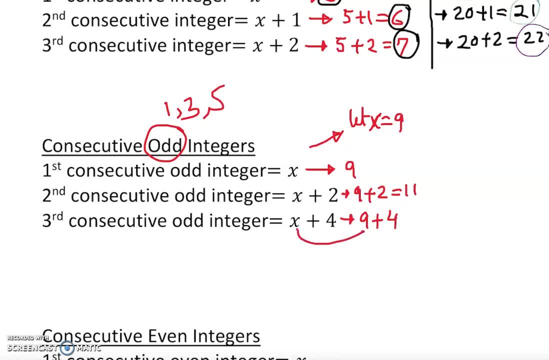 up with all those nine. so i'm assuming- okay, let's use this- this x is nine and four is there. i just rewrite those four right, so that is going to be 13.. so guess what? you have 9 comma 11, comma 13, and they are odd number each time. you see, okay guys, i'm gonna have. 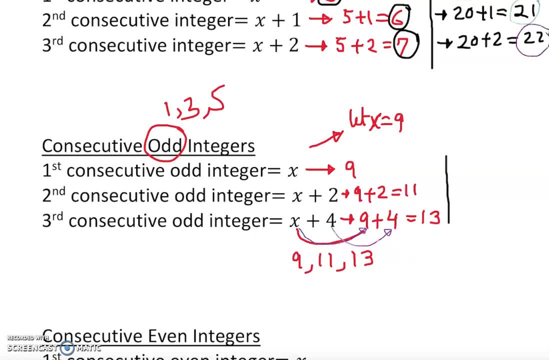 another example. i'm gonna ask someone to give me another example here. okay, um, please give me a number. okay, what you're saying? what 11? okay, just keep 11, x equal to 11.. so you're assuming x equal to 11.. so i'm going to actually put that here. you said x equal to 11.. 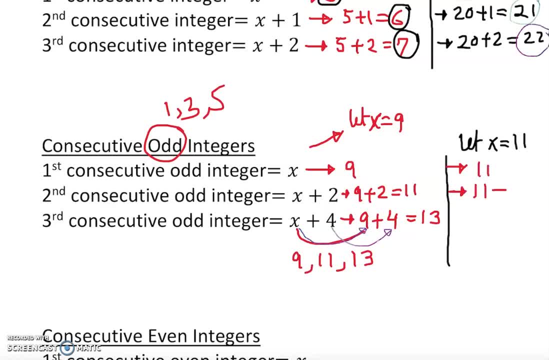 okay. next one is x equal to 11 plus 2, which is 13, okay, and then 11 plus 4, which is 15.. so, guys, no matter what you do, it gives you basically like: this one is 11 comma, 13 comma, 15.. they are basically odd integers one after another. so that makes sense. now i'll make. 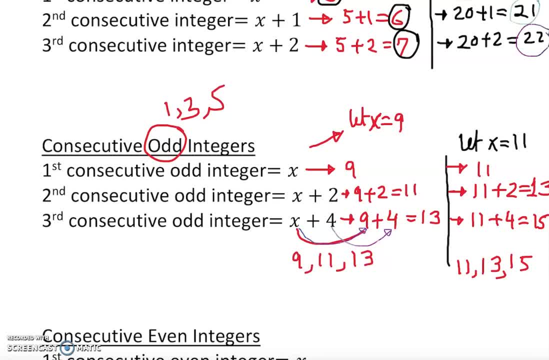 sure, guys, the second number is not going to be x plus 1.. second number: you always you should start x plus 2, x, you know. third, x plus 4, except it consecutive integers, if they say odd, or even down. here i'm going to show you. 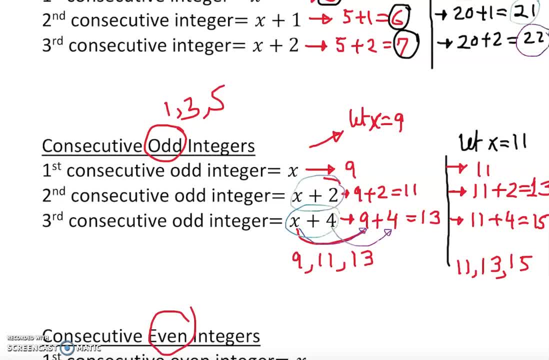 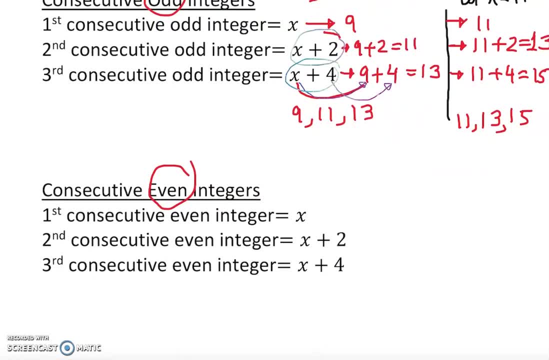 you basically do the same thing. it's basically same thing. let me show you here now you we are talking about. if the if question asks you find two consecutive, even integers, whose sum is this and that? okay, so first thing, you have to know how to write down first, one and second. 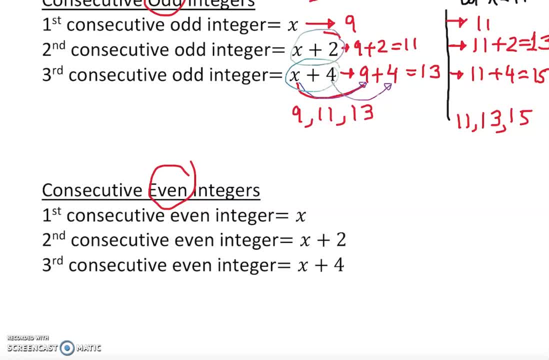 and third one. so this is how you do order. even is basically same way, while some you say: how come then we get odd? and even so, give me, let's have an example. let x equal to well, since we are doing even integers right, give me an even number, please. any choice what? eight, okay, someone said eight okay. 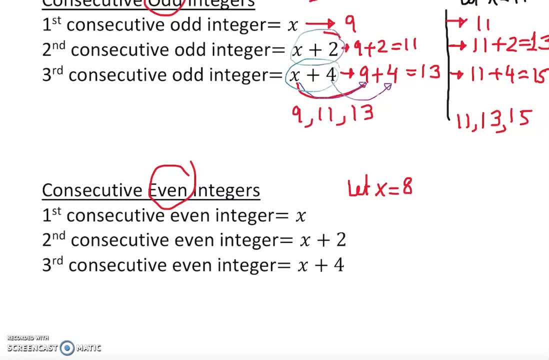 so let's start with eight. so i'm going to actually put down here x. well, let's do this red color in here. x equal to eight. you just said eight. then i'm going to have eight plus two, which is ten, and then i'm gonna have eight plus four. i have twelve guys. what is happening? look? 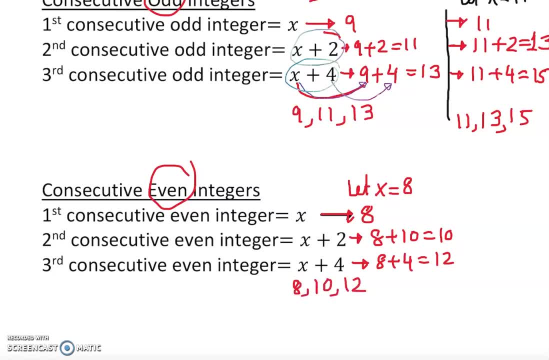 eight, ten, twelve, and all of them are even numbers, even integers. you clearly see that, right? i'm gonna have another example, so you are completely clear about this: consecutive integers, okay. so next one: you're gonna give me a number, let x equal to in this case, what i'm gonna make up? one, i'm gonna make up with the easy one. okay, just number two, i'm assuming. 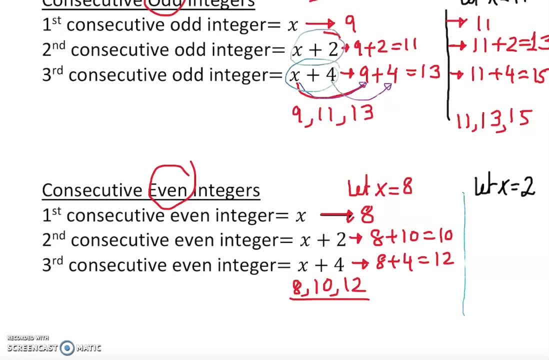 this number two is my, even integers, or you can come up with number. 200 still is going to be same thing. okay, you know what? let's make it 200 with big number. you should see big number, right, okay, so first one is 200, second one is 200. 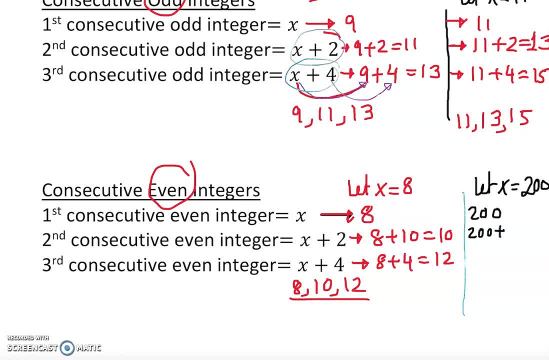 plus 200 plus two, that's two hundred two, and the following one should be 200 plus four, so two hundred four. guess what? all of them even 200, 202, 204, and all of them are even integers. that's how you deal with, that's how you deal with consecutive integers, and also that's. 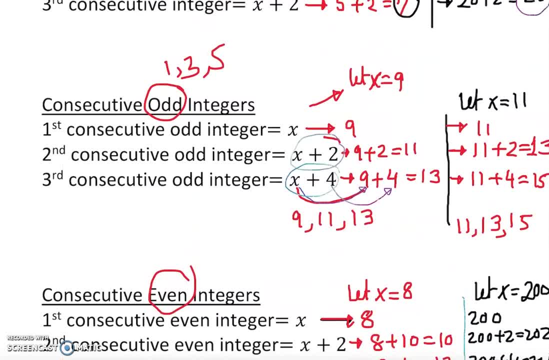 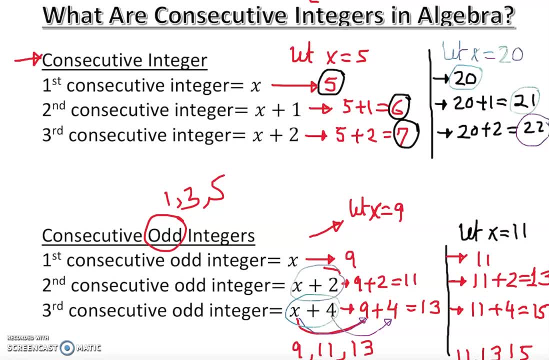 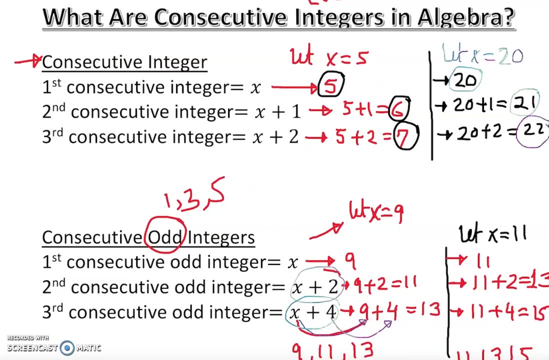 know that they're going to give you nice outcome as question ask you. so you have to know first, second, third, at least, and you go further. you look for more. so what we learn from this discussion here? look at these guys. we learn that once question asks you to find three consecutive. 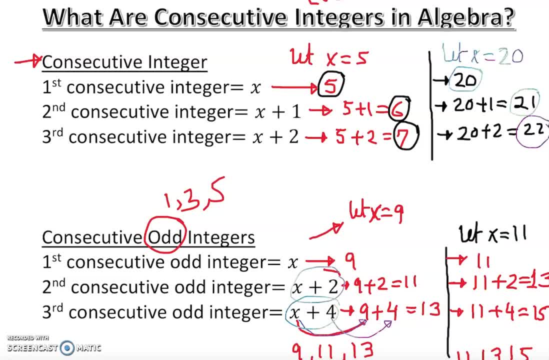 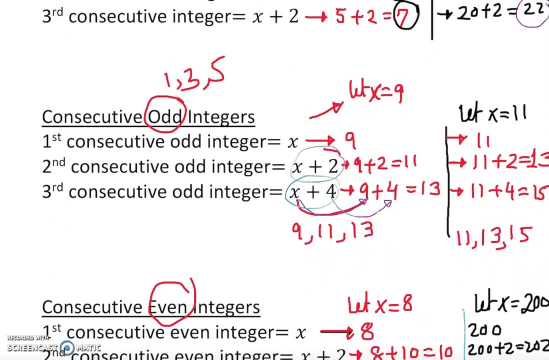 integers. we just come up with like this: x first one, second one is x plus two, third one is so: second one is x plus one, third one is x plus two. you just, you know, go down here easily without any interruption. okay so, and the next one is basically odd, odd, and even there is a similarity. 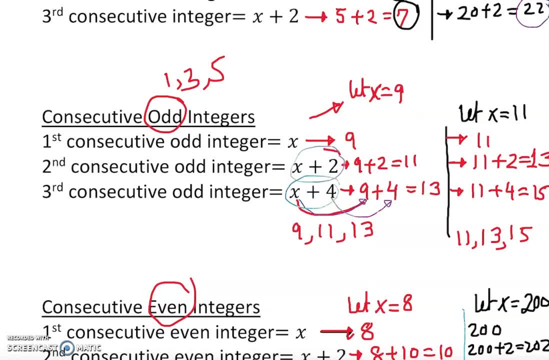 you use the same thing, basically, okay, x. second one is x plus two. third one is x plus four. if there is a fourth one is going to be x plus six. both of them, okay, and that's all. that's how you deal with it, thank you. 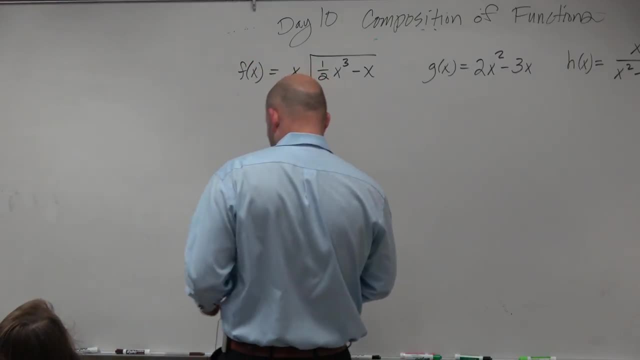 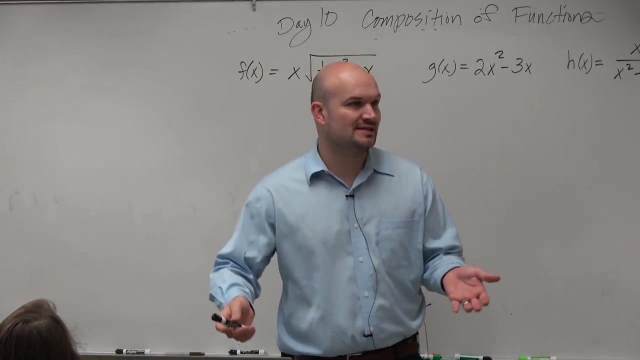 Ladies and gentlemen. so when you guys take this quiz that's going to be coming up next class period, one of the things that you guys will notice is giving me the answer is not what I am looking for. I do not care about the answer- correct answer- I care about the process of you working through it. 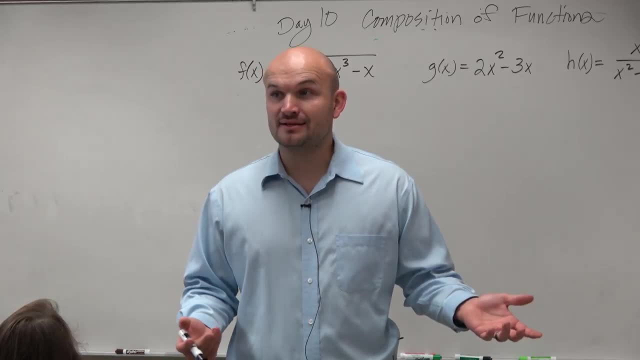 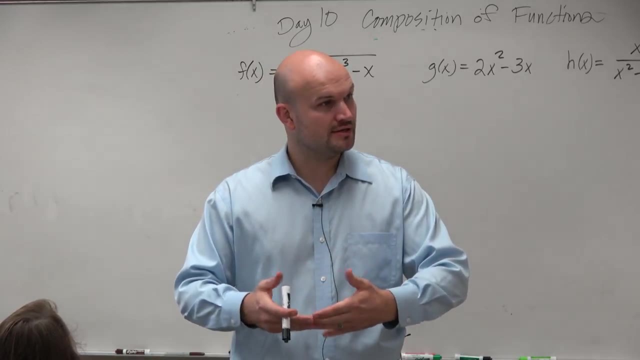 So just writing in odd or even, and just making a stab at it- because you really have, you know, one third of a chance of getting it right is not going to count, worth any points Showing me the steps and the work will definitely work okay. So you're not going to have a. 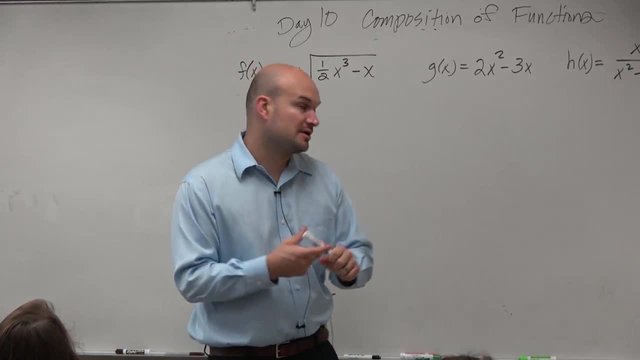 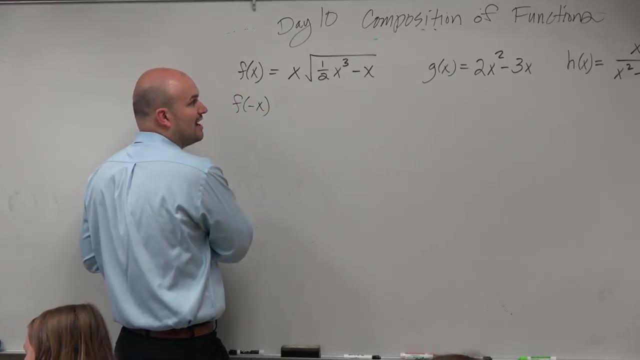 calculator. So just looking at the graph and saying hey, it's even odd or neither is not going to work. You are going to have to show me that you can identify, And the first thing you're going to want to show me is: I can evaluate this function for f of negative x. So when you replace 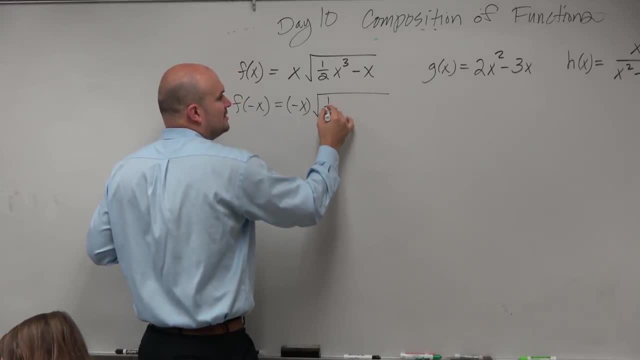 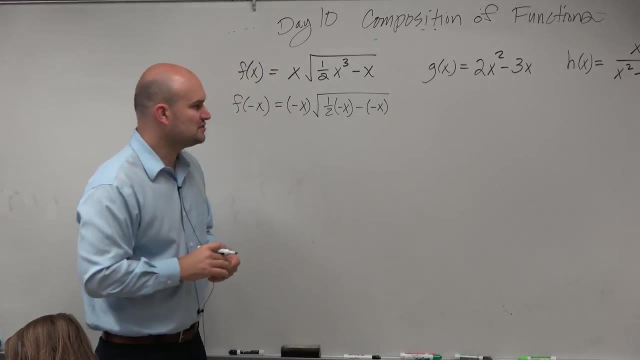 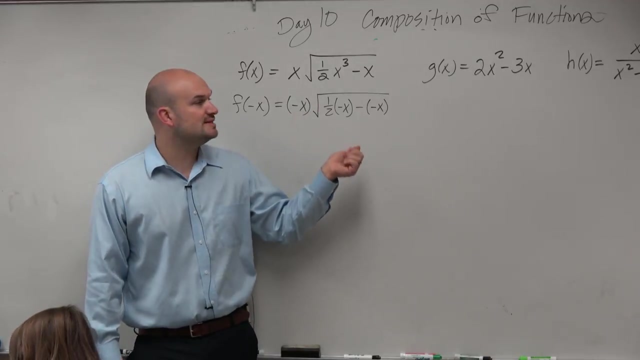 again notice how I'm using parentheses to represent that I'm inserting in a value into my function. This is really important because people- again, this is where the mistakes happen- People don't use parentheses and they don't don't put in a minus, a negative x, because that really turns into a positive x, right. 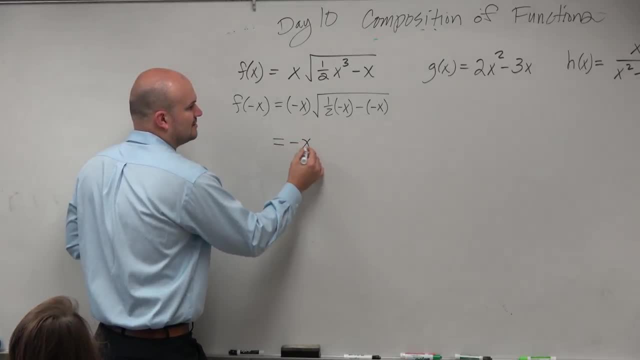 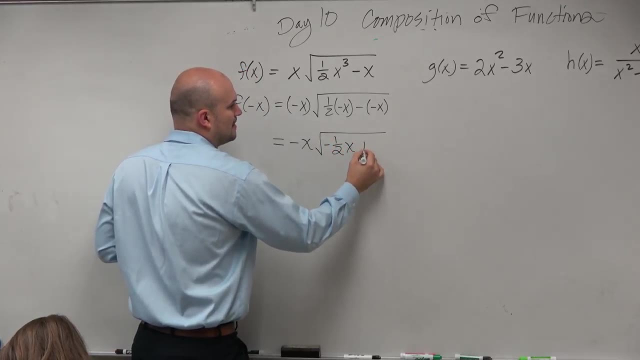 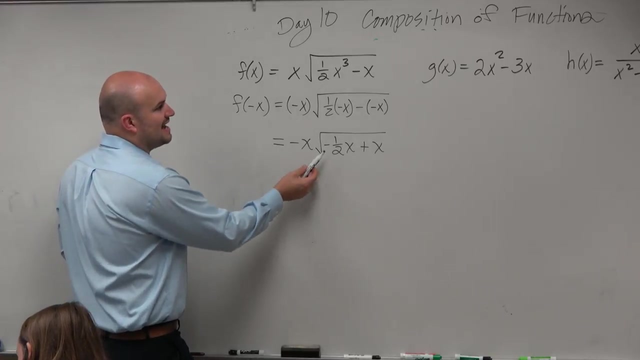 So, anyways, when we go and take a look at this, we have negative x, square root of negative one, half x plus x. Would you guys agree? Yes, Okay. Now is that taking me back to my original function? No, Okay, So let's check to see if that is the opposite of the function. 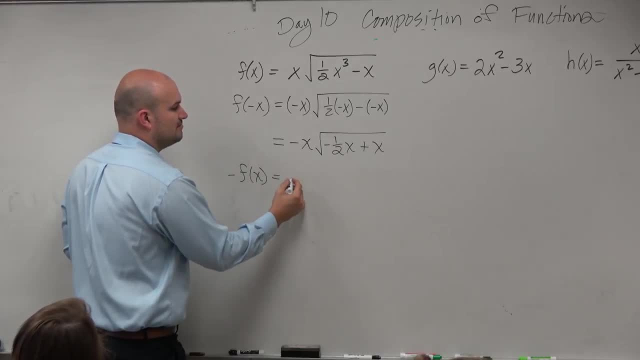 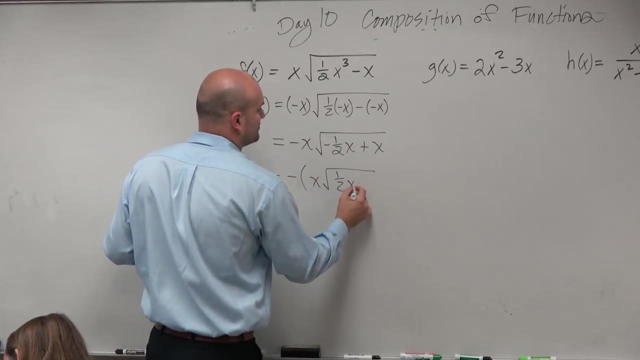 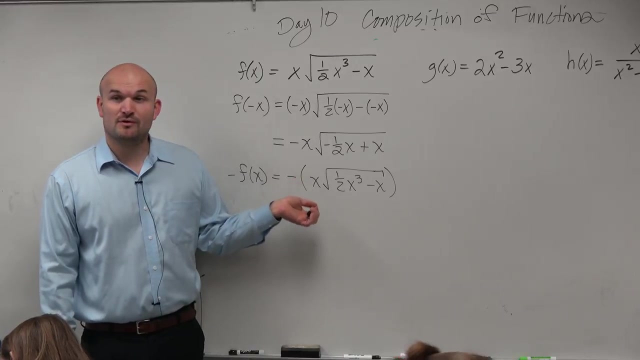 Now, here again, we have to be really careful When we're multiplying our function. we need to remember what the operations are with square roots, And this is where I actually forgot to mention. Can we take a number outside, a radical, when it's not having multiply it inside?